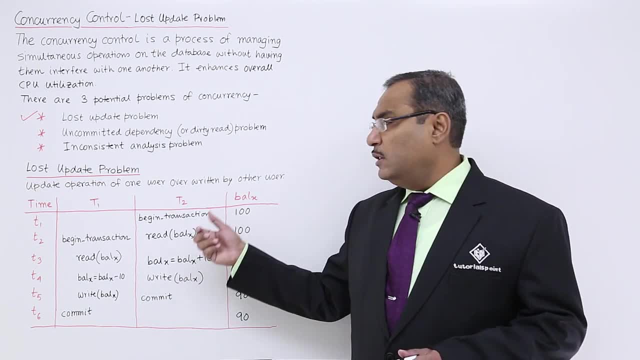 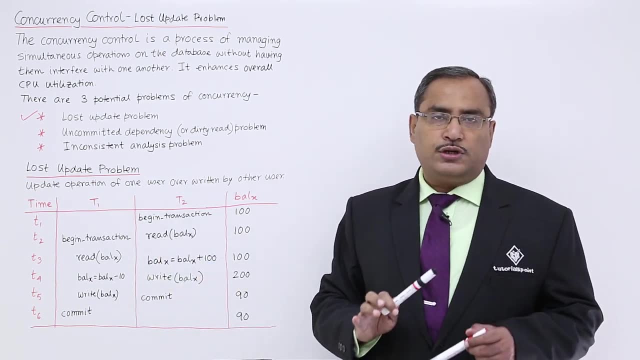 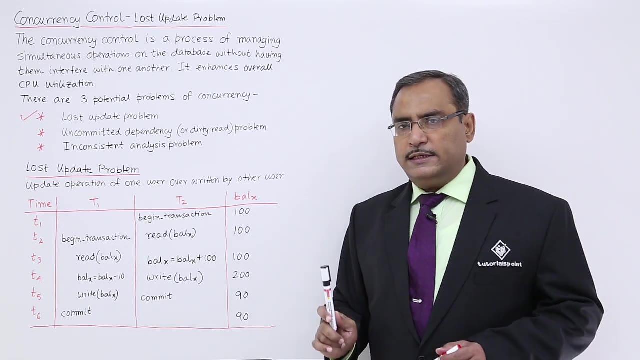 T2.. So the updates which will be done on the variable balance x by T2 will be overwritten by the transaction T1.. So that is our lost update problem. See. So here begin transaction read balance x. Initially the balance x value was 100. So 100 has been read At T3 instant. 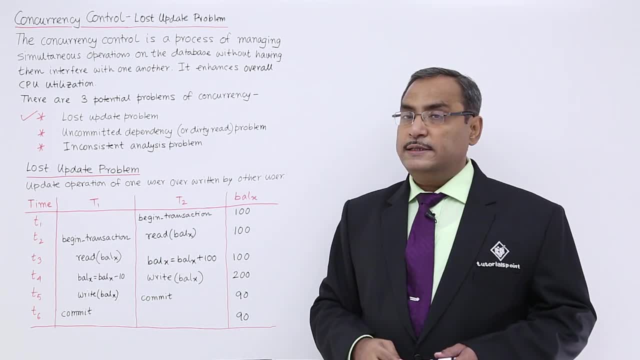 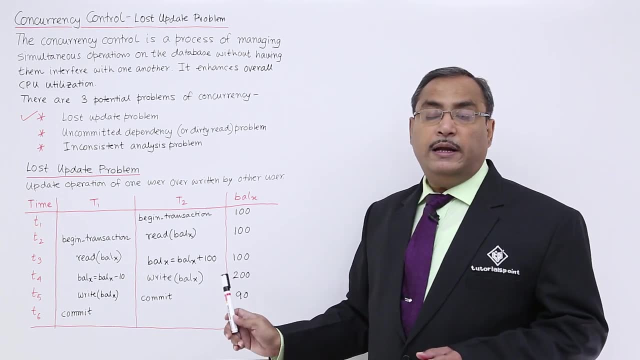 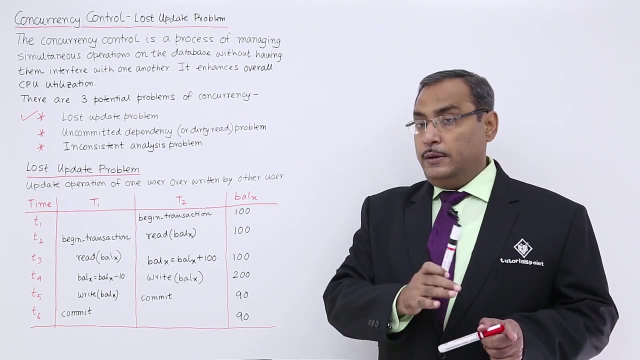 balance x is equal to balance x plus 100. So the balance x has become 200 here. but here I shall not write 200 under the column head balance x, because only the variable instance in the memory has got updated to 200, but it has not been written back on to the database. 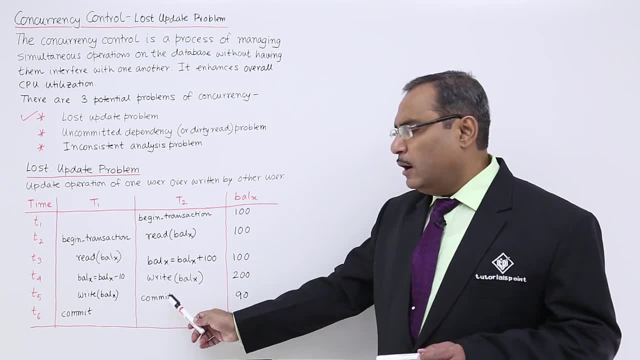 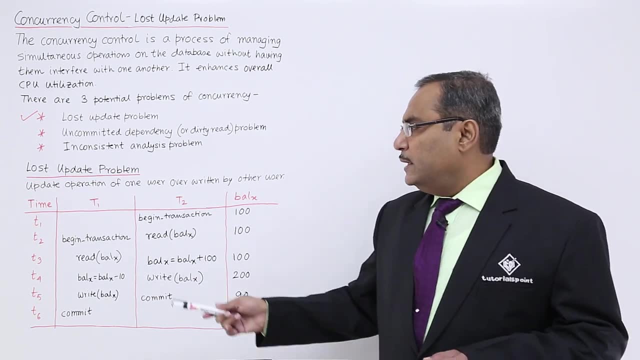 So now write balance x- now it has become 200- and commit it will make the change permanent. So that is the purpose of transaction T2, which is the older transaction. So this is the older transaction, Say in the younger transaction T1.. So begin transaction at T2. 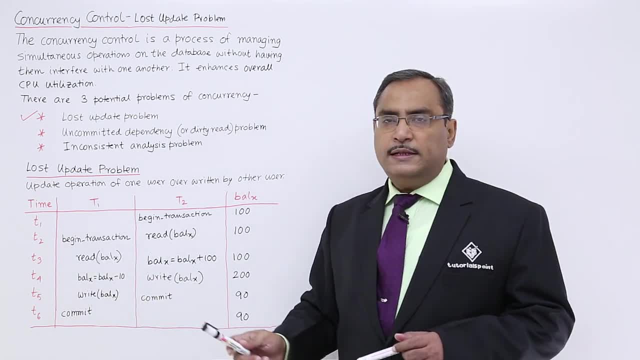 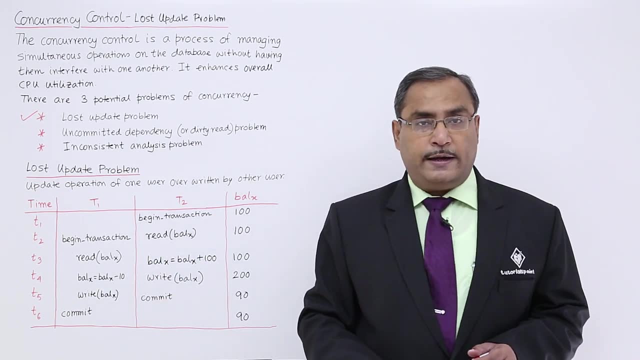 instant, and now at T3 instant we are having this read: balance x. So the current balance x value is 100.. So 100 has been read, Balance x has been decremented by 10, but I shall not write 90 here because it has not been written yet. Now write balance x will make. 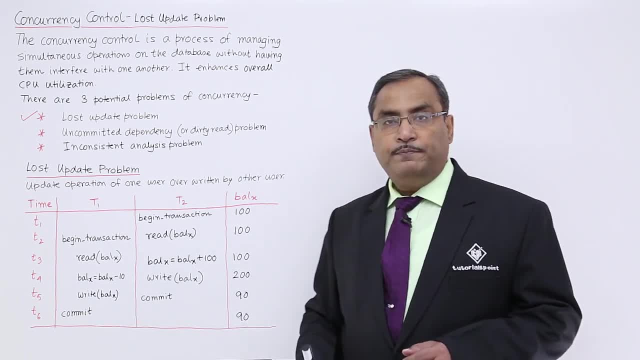 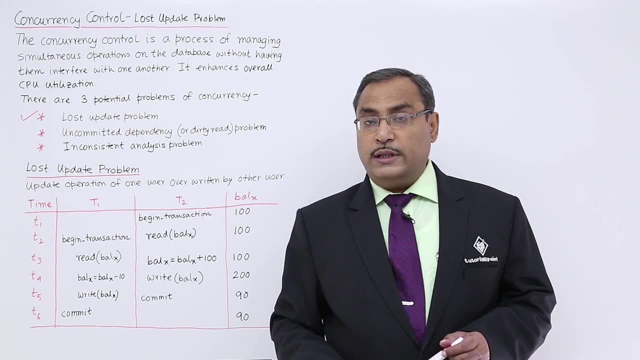 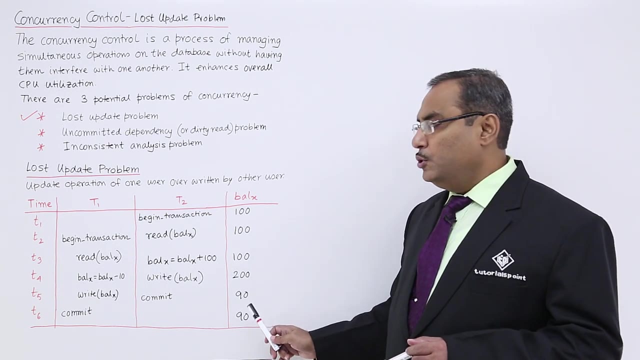 that one, 90 and commit will make the change permanent. So now what is happening? You see, There is no concurrency control between T2 and T1. So that is why 100 has got updated to 200 by T2 and same 100 has got updated to 90 by transaction T1. and that is the problem. 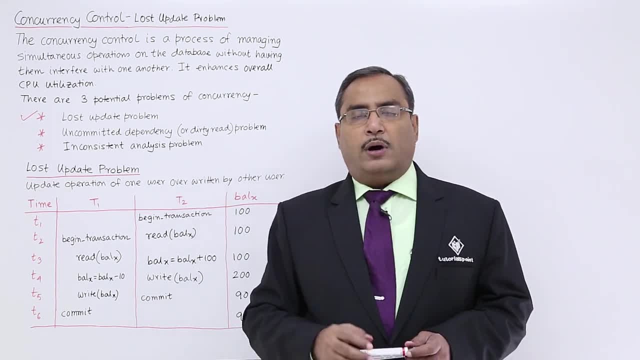 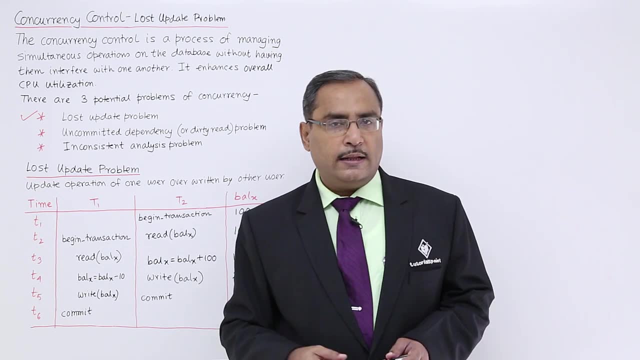 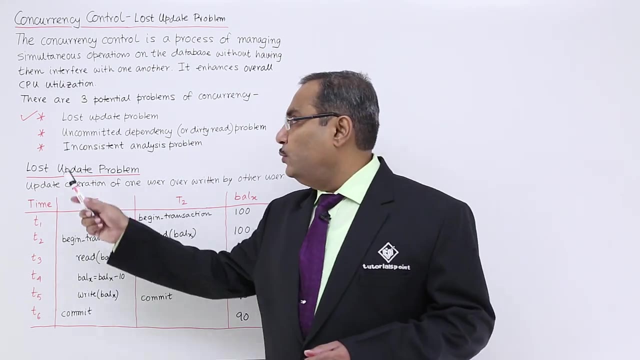 known as the lost update problem. So update of one transaction, update of one user, will be cancelled out by the update carried out by the another user. So as that is, no concurrency control here occurred. So in the next video we shall be going for uncommitted dependency problem. So 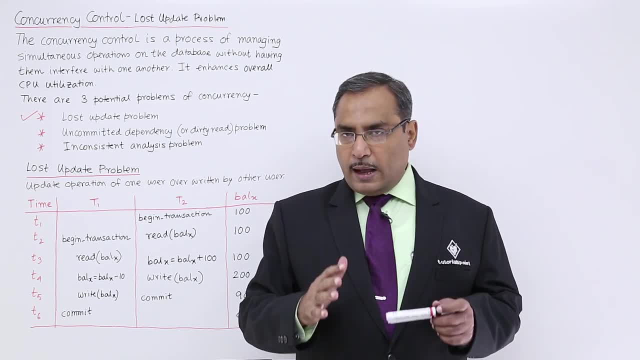 please watch next videos to have the continuation and to have the knowledge over this concurrency control. Thanks for watching this video.